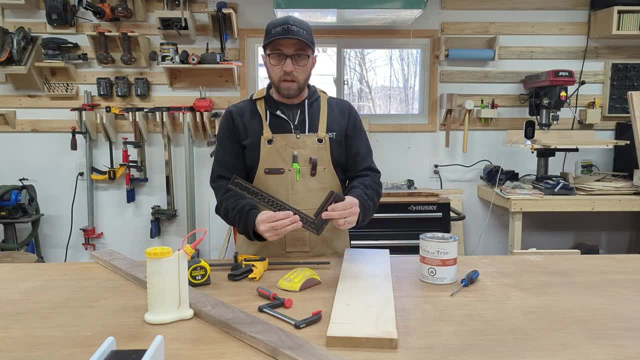 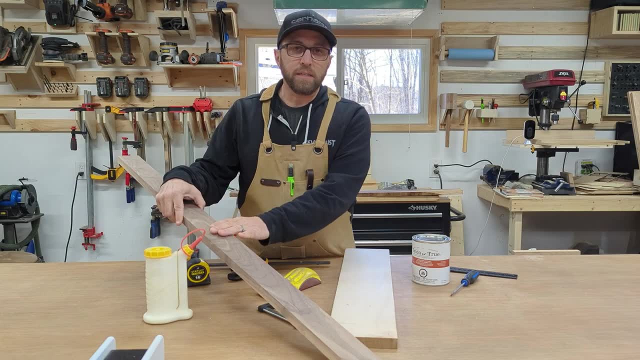 your piece For today's project. all I'm going to be using is: I've got a square here to make sure that our edges are going to be at a 90 degree angle. I've got a piece of walnut left over from a project. I've also got a piece of maple that's left over, so we're going to be ripping that down. 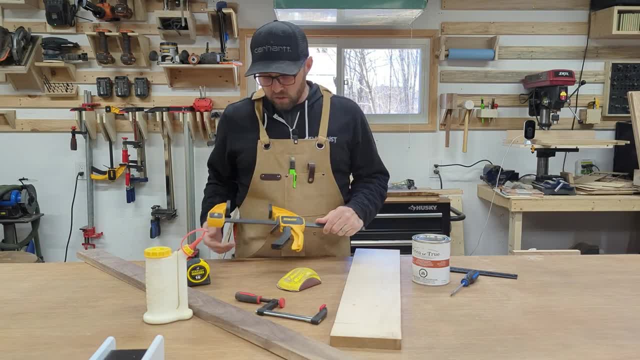 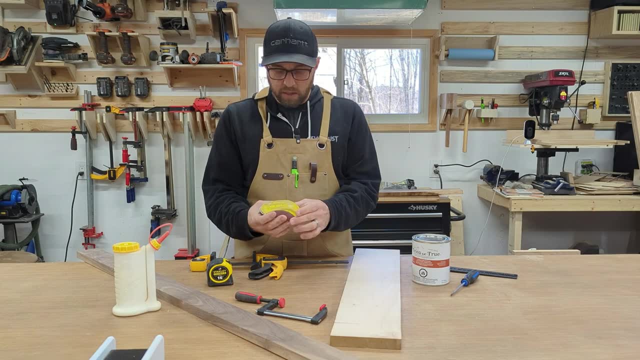 for our project, Some clamps that I'll be using as well for our glue-ups- A tape measure, of course, to measure everything We've got our glue here I've also got and I don't for this project here. 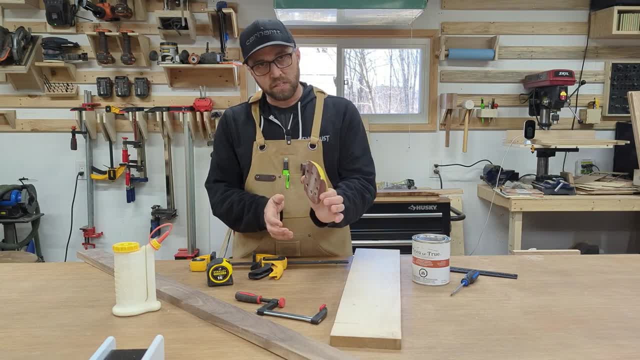 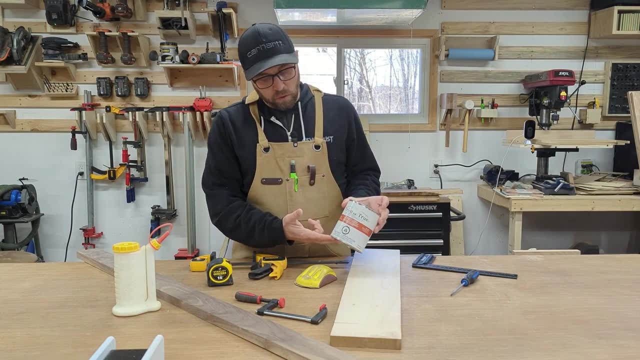 I'm going to do probably the bulk of the sanding by hand using this little sanding block. I'm going to put a link to this little block in the description where I purchased it from. Then we're also going to be using this here, which is a tried and true linseed oil and beeswax. 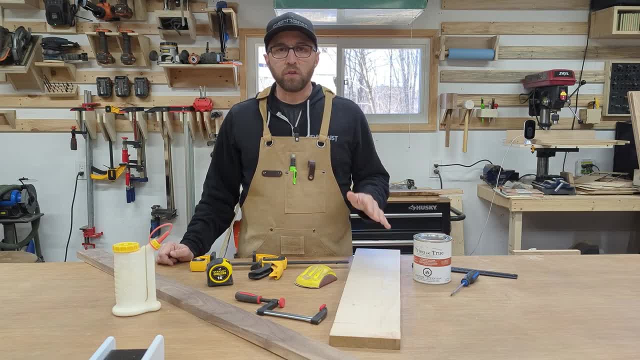 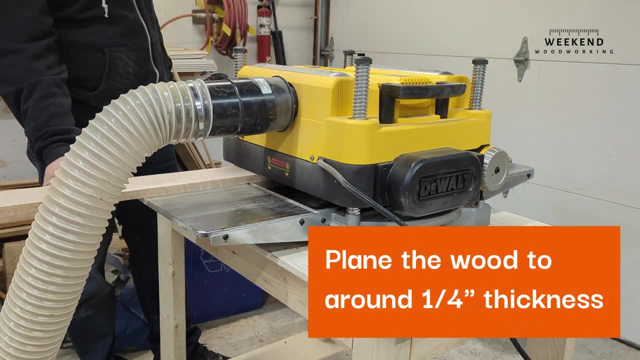 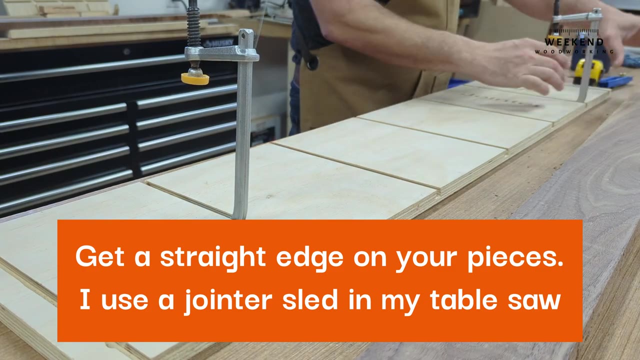 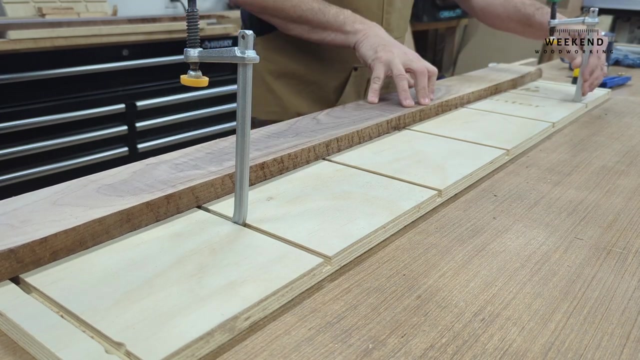 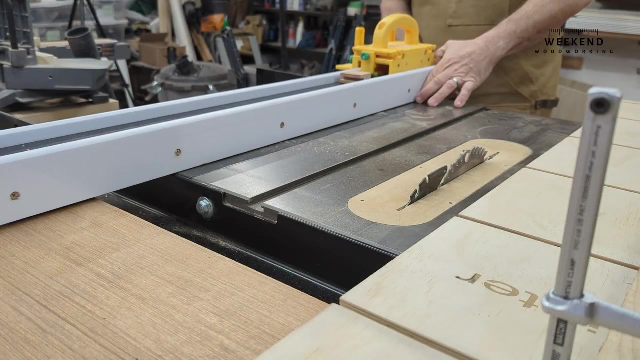 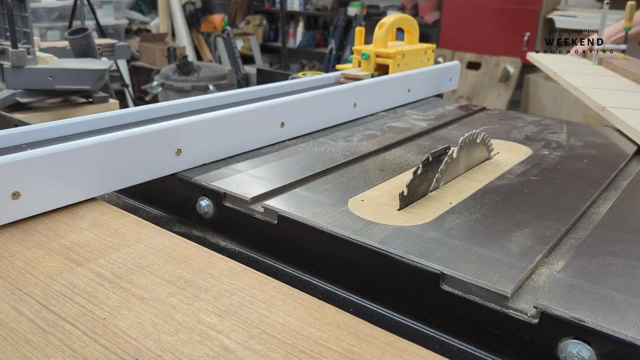 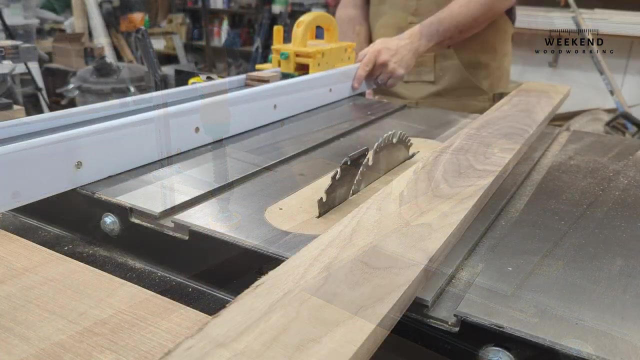 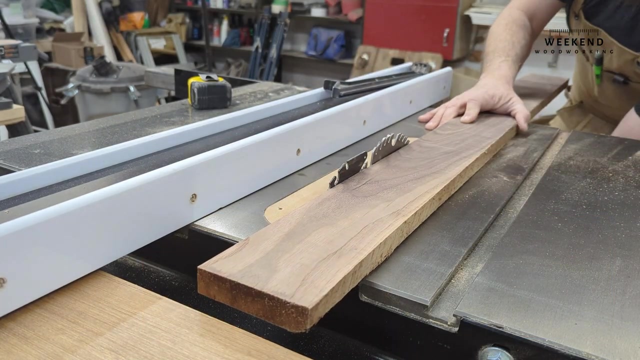 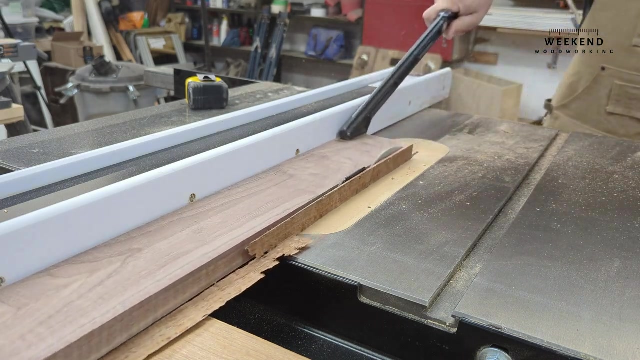 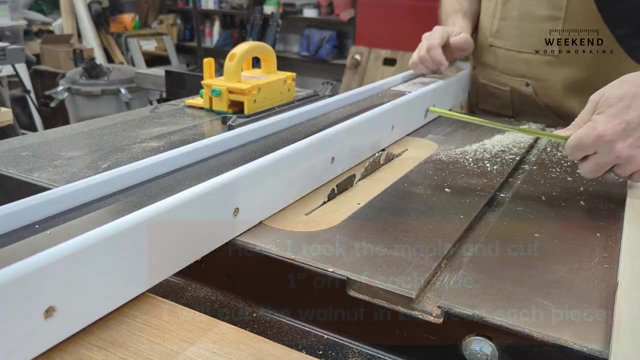 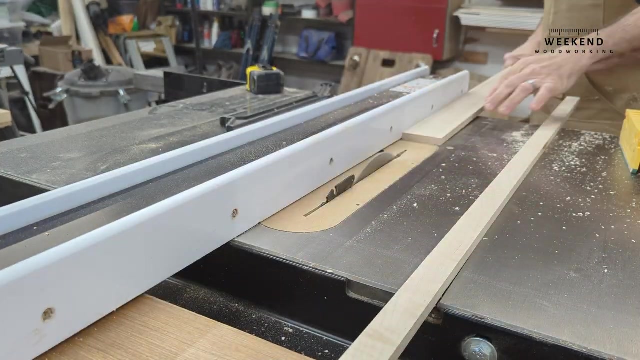 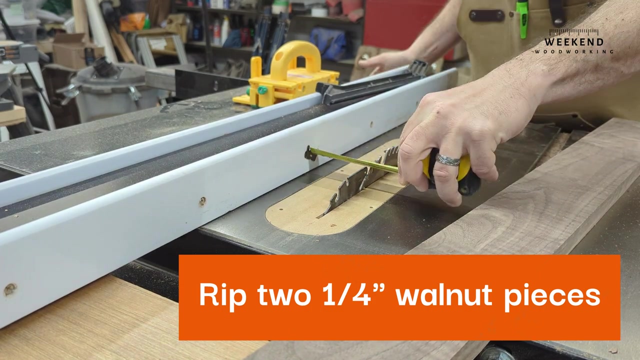 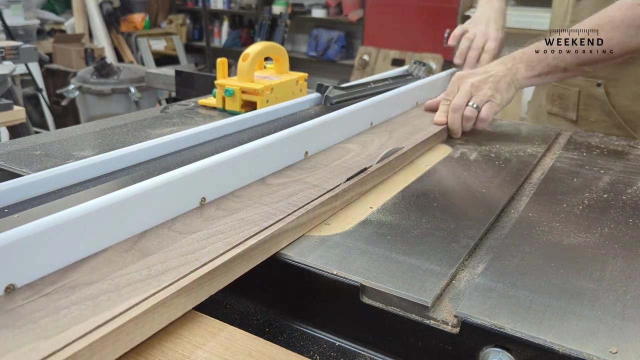 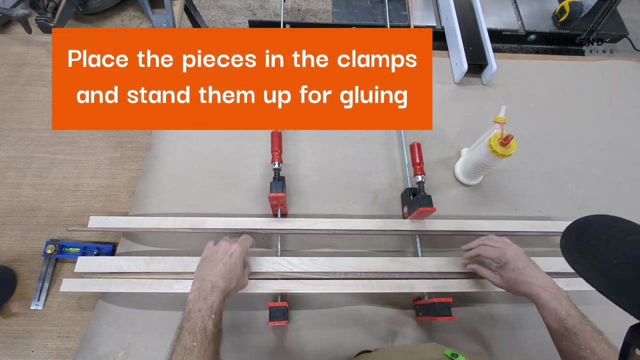 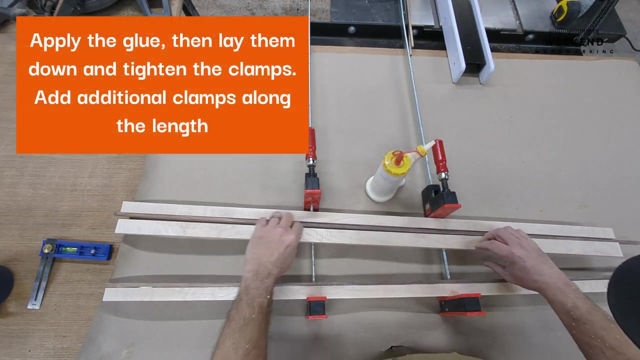 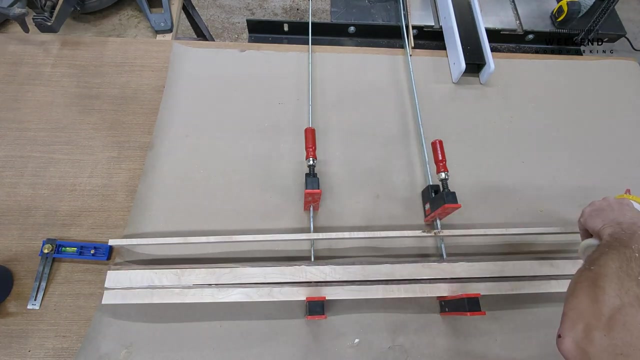 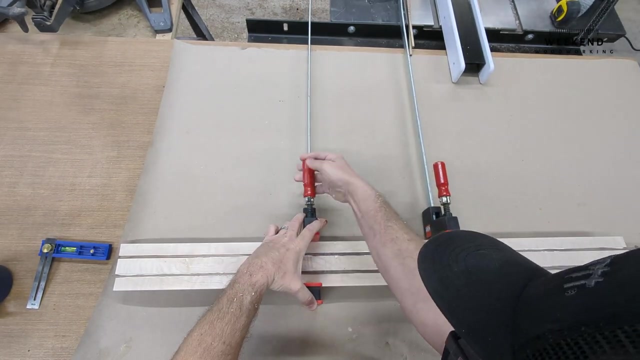 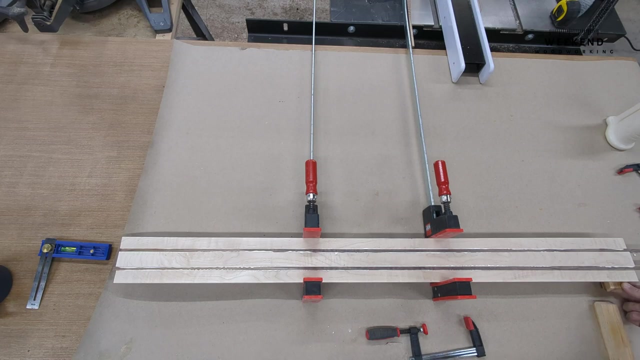 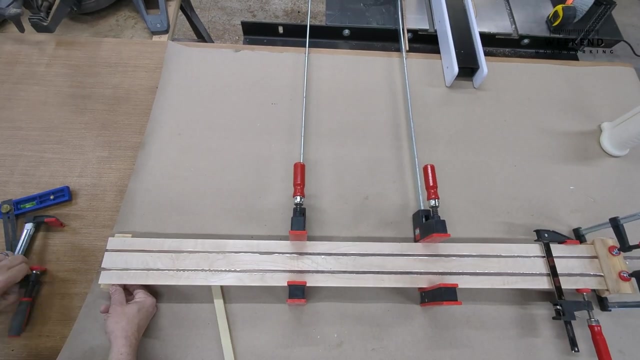 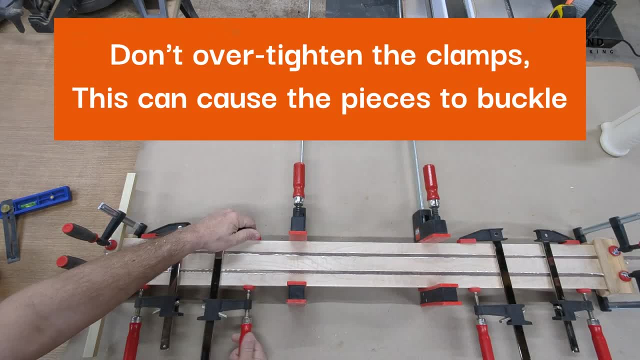 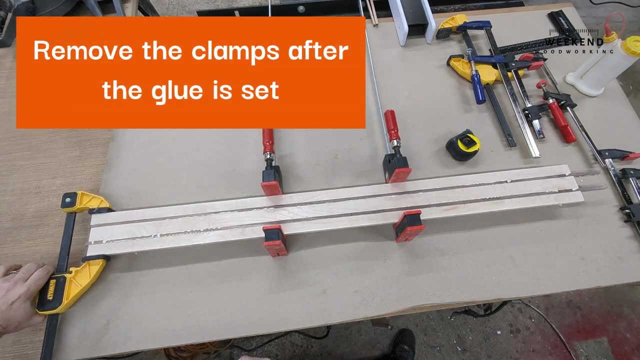 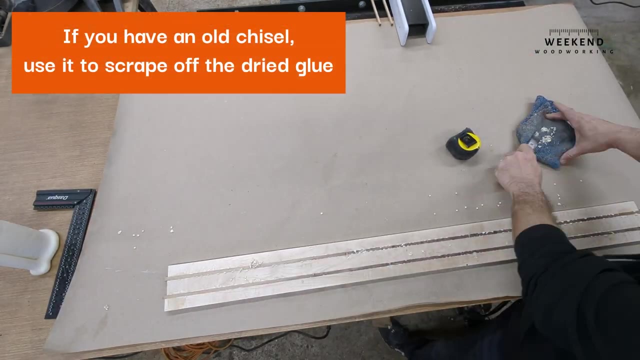 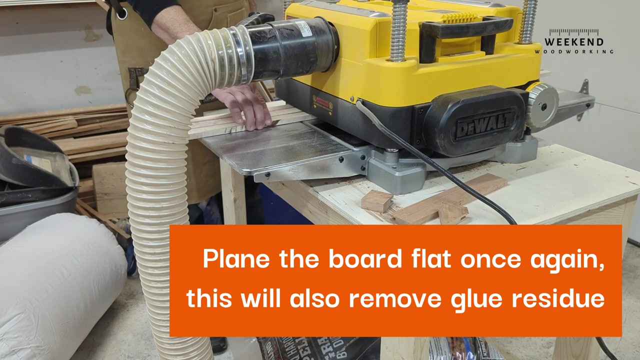 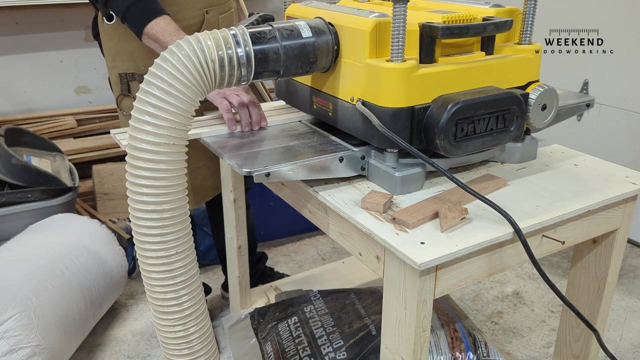 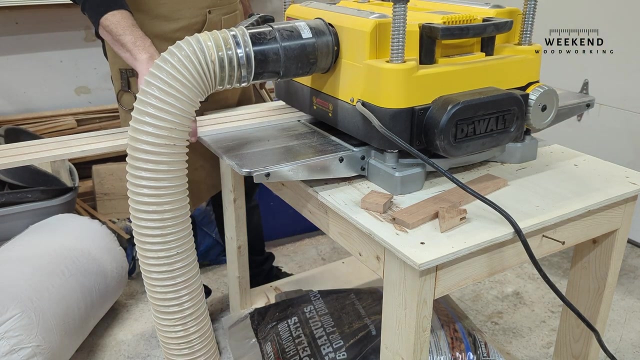 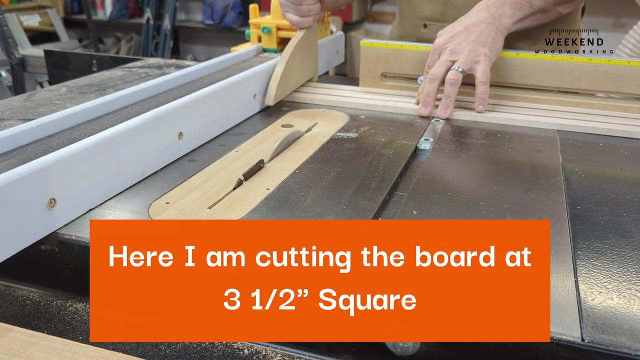 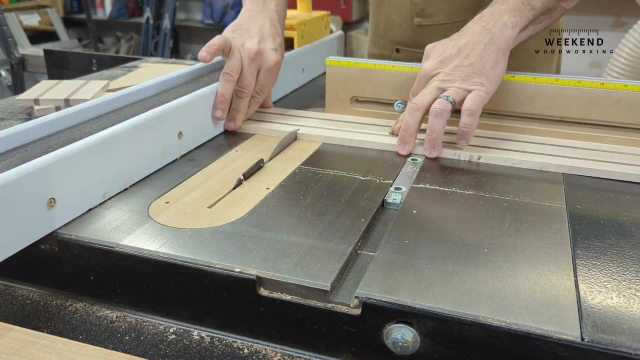 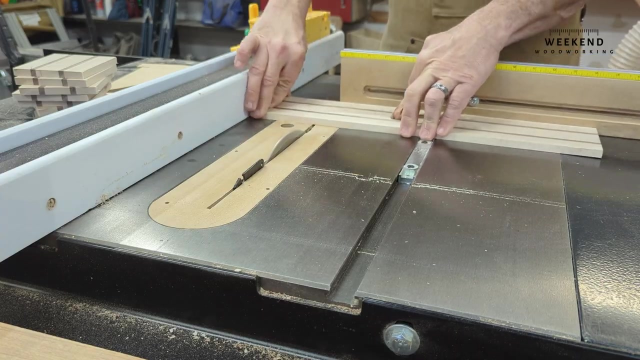 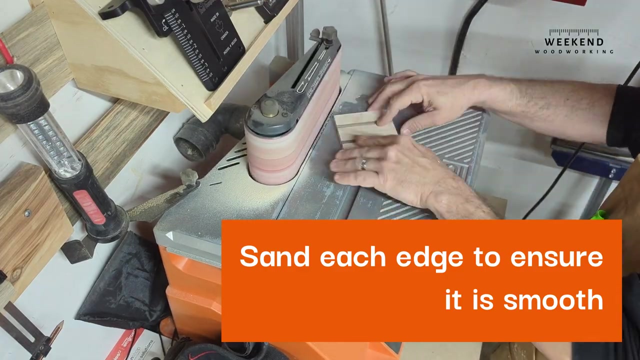 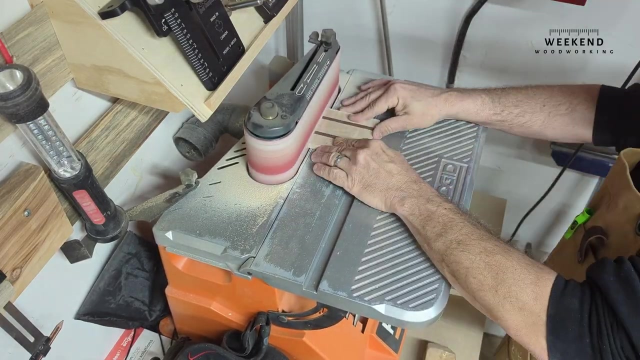 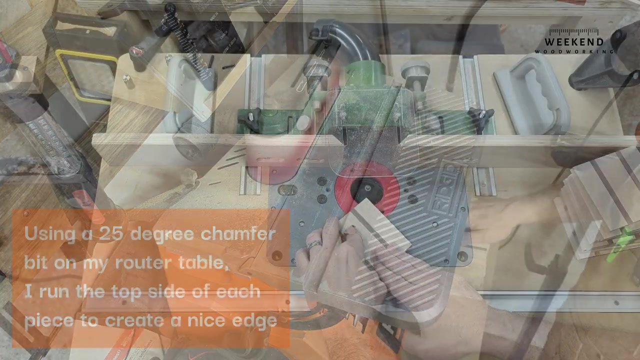 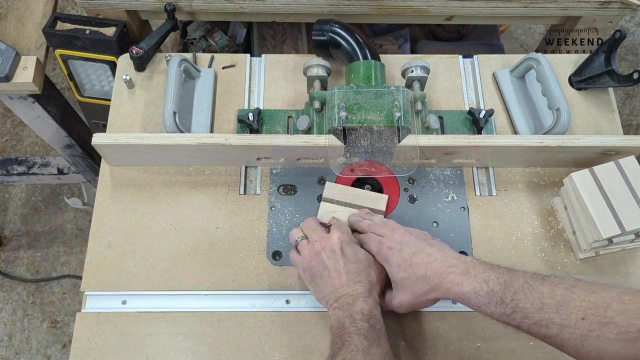 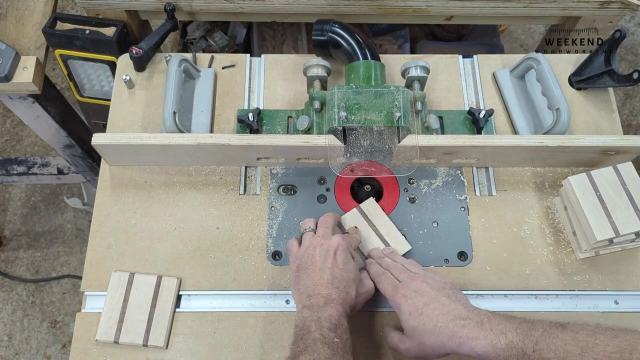 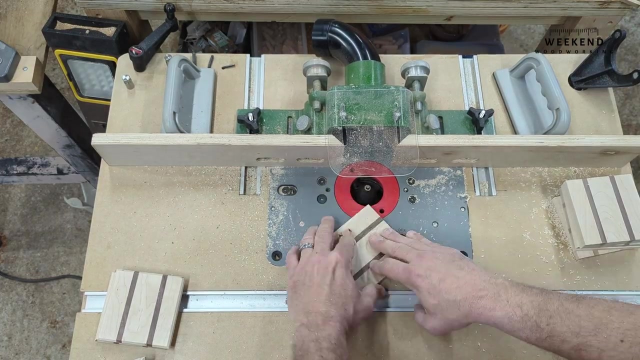 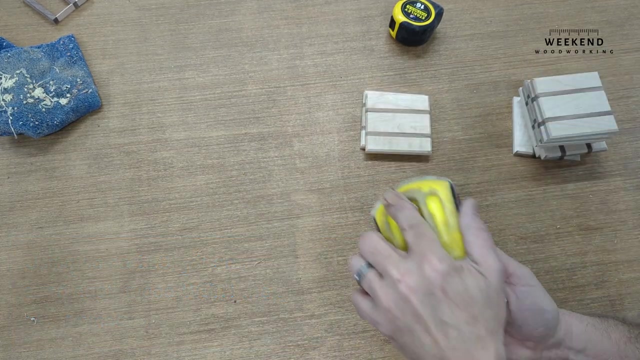 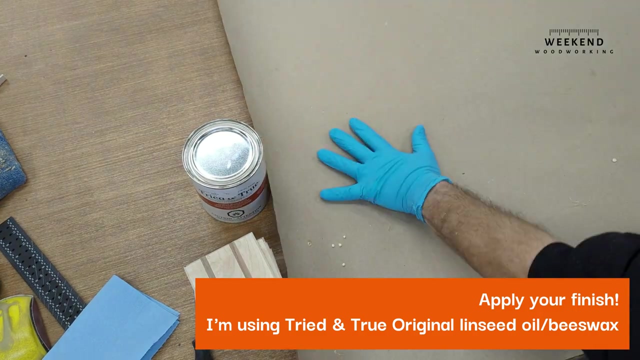 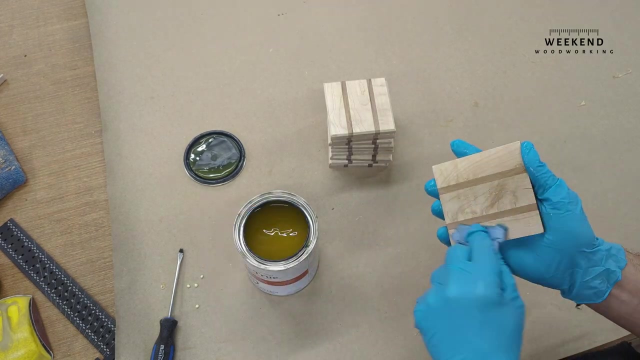 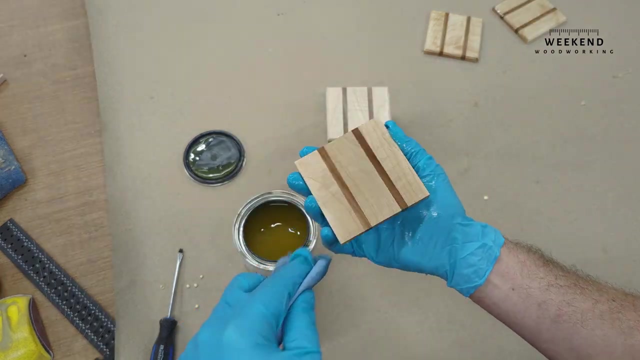 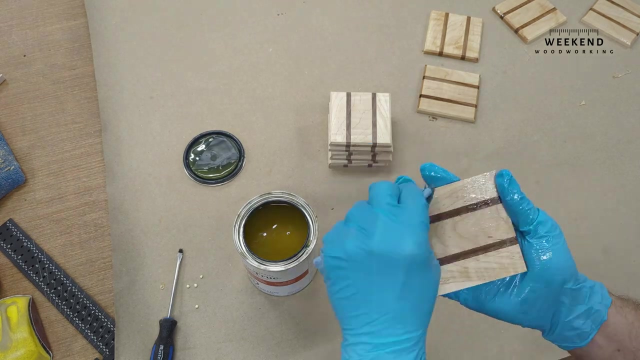 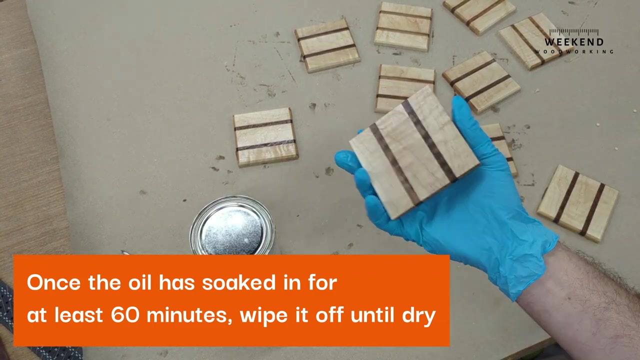 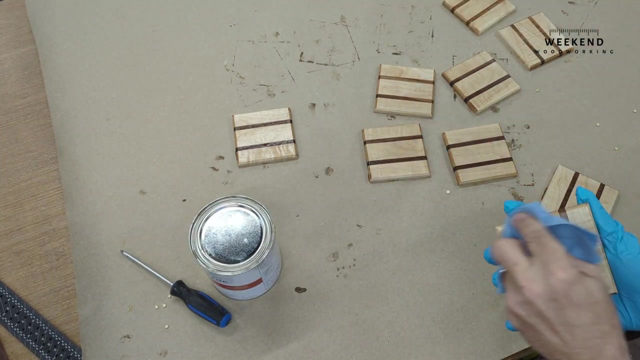 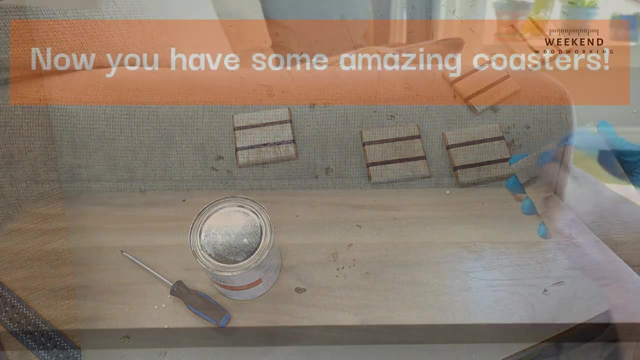 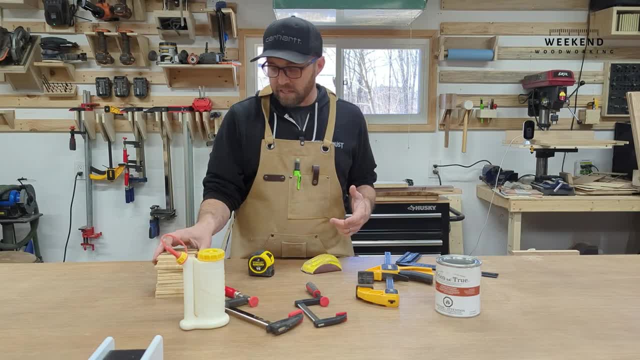 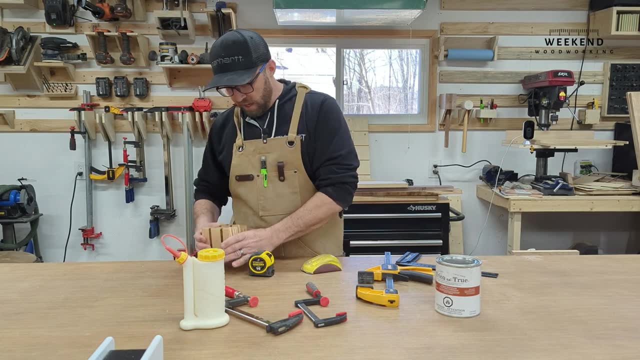 All right, so let's get into it. Well, I'll take you off screen here. Well, I hope you enjoyed our little build video of making some of these really neat little coasters out of maple and walnut. There's not much to them, and then they were just finished beautifully and you can see that little bit of a sheen that comes. 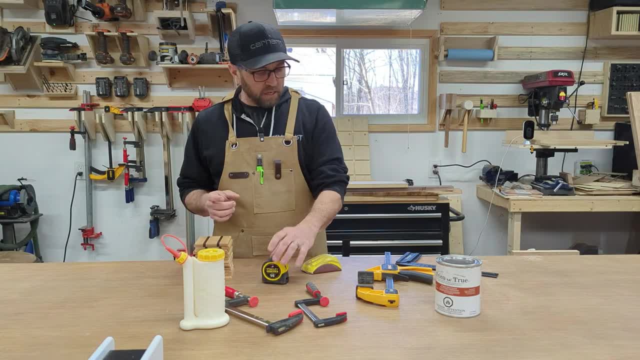 out in the maple wood grain, that the maple wood grain That comes up right there behind the one that's growing a bit right there behind the one that's growing a bit right, because of our tried and true linseed oil and beeswax finish, which was really nice.